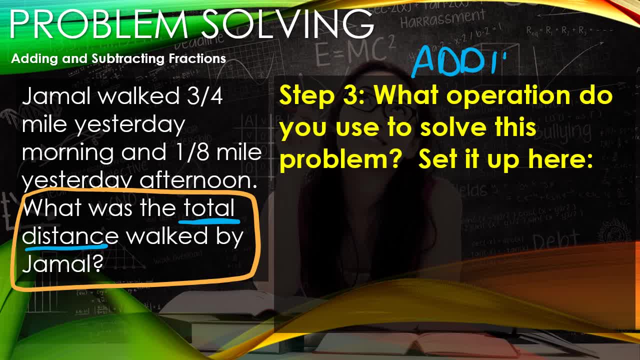 problem is: you're almost halfway there in solving this problem, And so we can look at the question again. We are adding friends, We're going to be adding these two fractions together, And so we're going to go ahead and set that up in this box in step number three. So we're going to set it up as three. 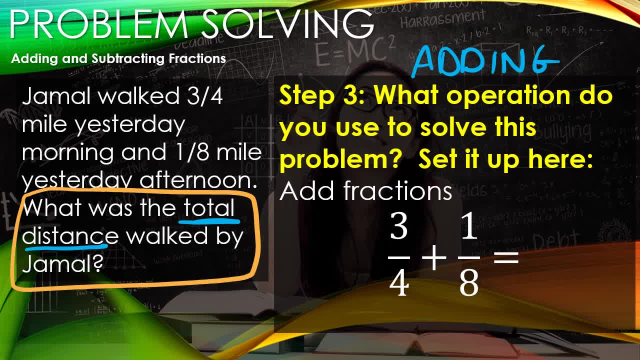 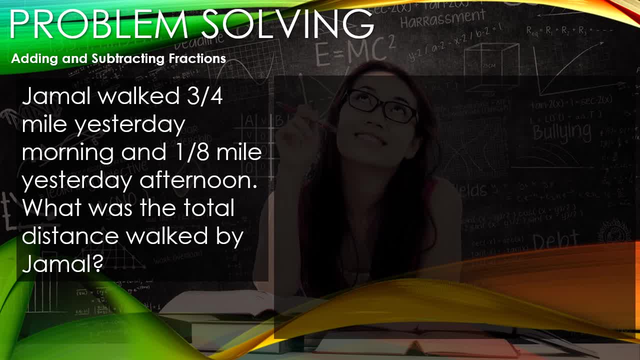 fourths plus one eighth. So you can see we haven't solved anything yet, but we're just setting ourselves up to be very successful in solving this problem. So now we have to figure out what are steps to answer this question. We know that we need to make. 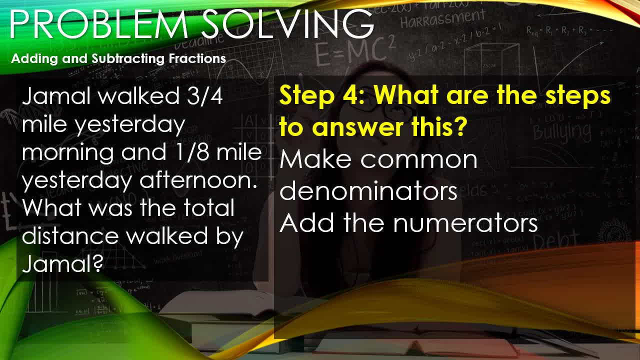 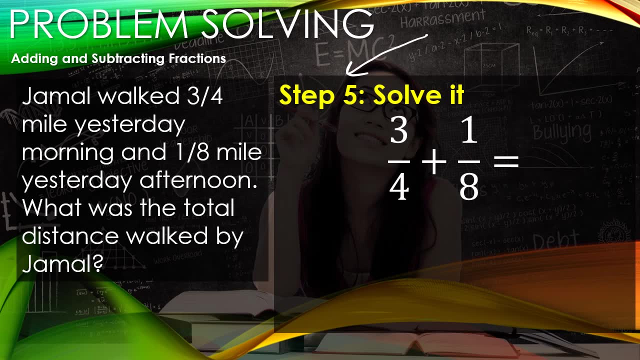 common denominators. first, We're going to add our numerators together, But we're going to keep the denominator the same. So whatever we made with common denominators in this first part, we're going to keep the denominators the same. So now we actually have to solve it. So here we go. Let's. 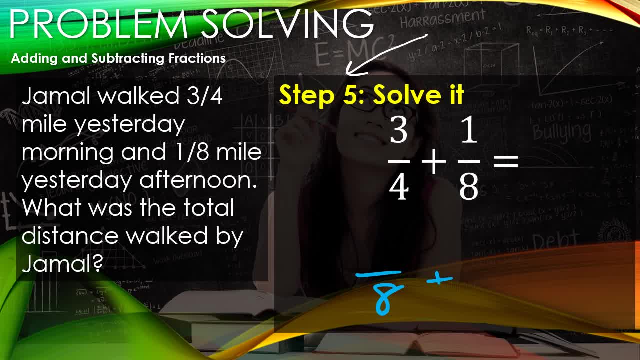 go and change three fourths. We need to have fractions that are over. eight is our common denominator. So for three fourths we're going to multiply the denominator and numerator by two. So four times two gives us eighths. Three times two gives us six. 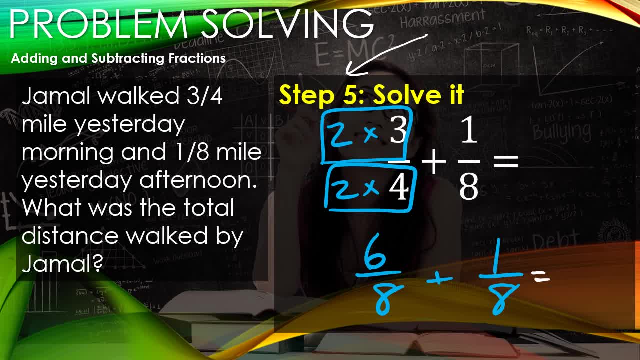 One eighth is already good to go, So we're going to just go ahead and add our numerators together. So six plus one is seven And our denominators, since they're common denominators of eight, that gives us a denominator eight, And so let's go and make sure, add our label in there. 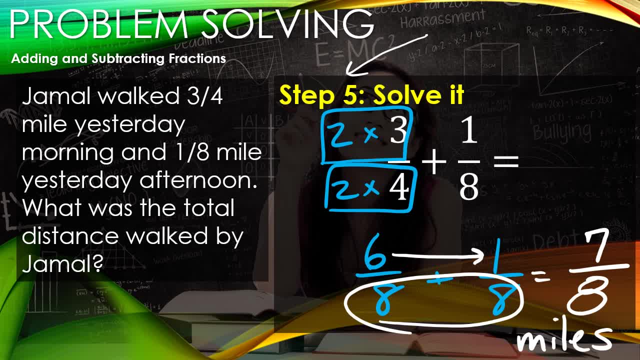 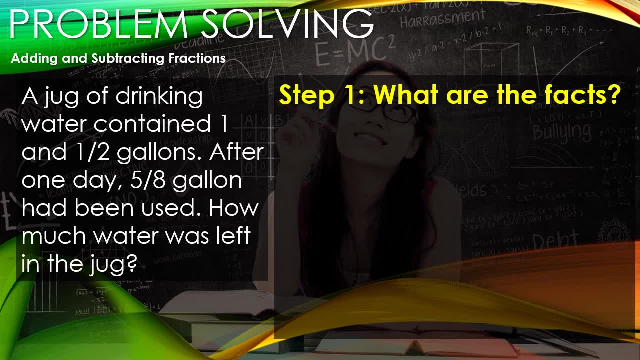 The label is miles. So we say our friend Jamal. the total distance he walked was seven eighths of a mile. So here on the back of the notes page we have this problem. We have a jug of drinking water contained one and a half gallons. After one day, five, eighths gallons have been used. How much water? 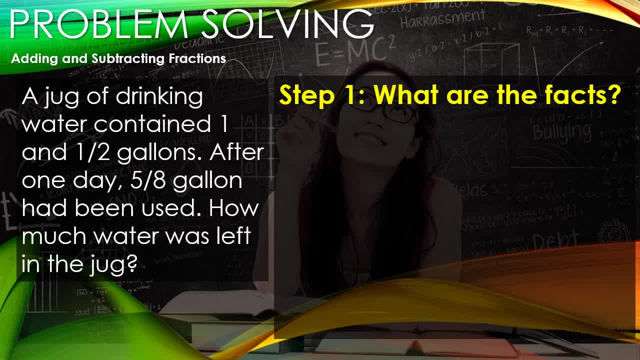 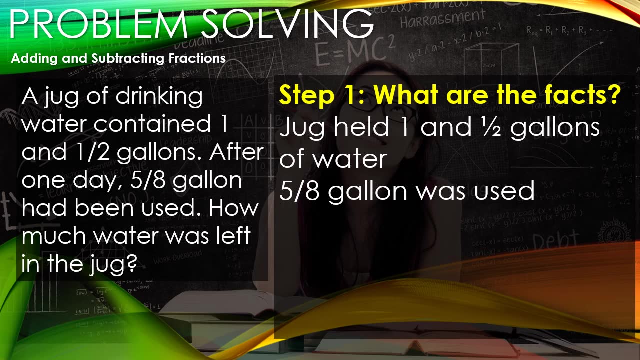 was left in the jug. So step one is: what are the facts? The fact is we had a jug that held one and a half gallons of water, that 5, 8 gallons was used, and so this might have been a sporting event with Gatorade container filled with water. this could have been. maybe they were on. 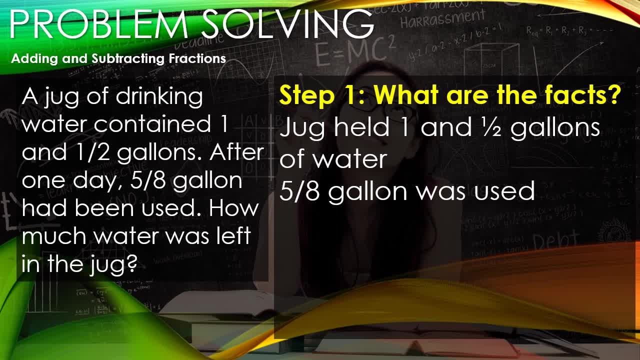 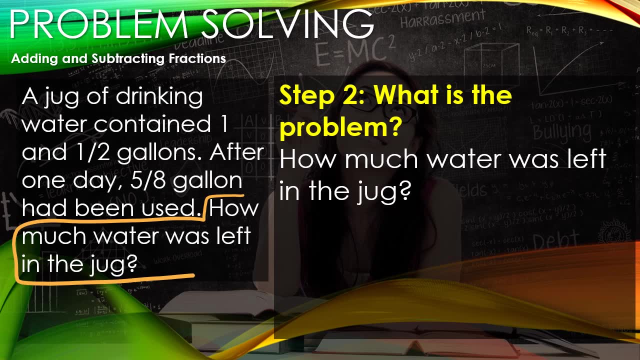 a picnic. maybe they were out camping, who knows? but this jug held one and a half gallons. 5, 8 was used. so those are facts. what the problem is, the problem is usually with the question mark: how much water was left in the jug, and so that's. 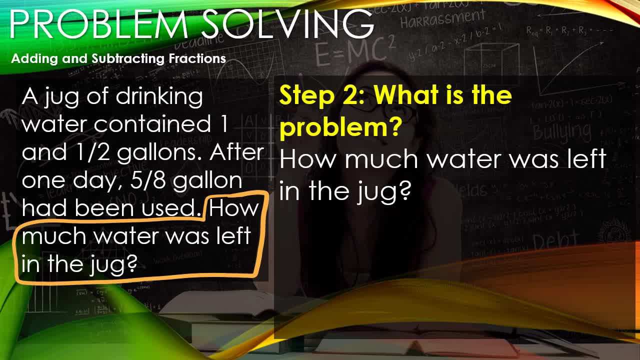 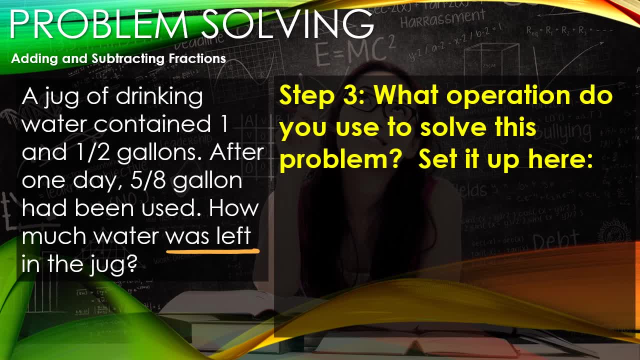 step twos: we're just figuring out how much is left after the five eighths was used. so what operation is this? so how much water was left? we'd say that we are now subtracting these fractions. so we're subtracting the fractions and we're just 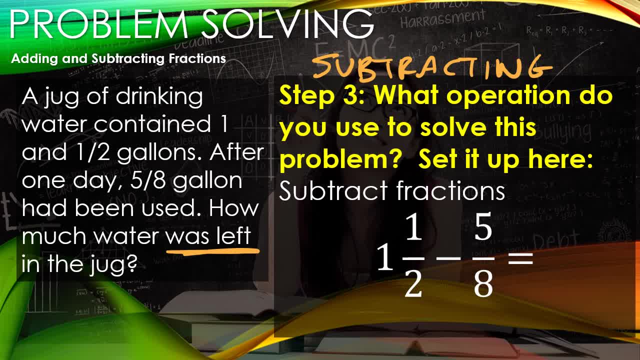 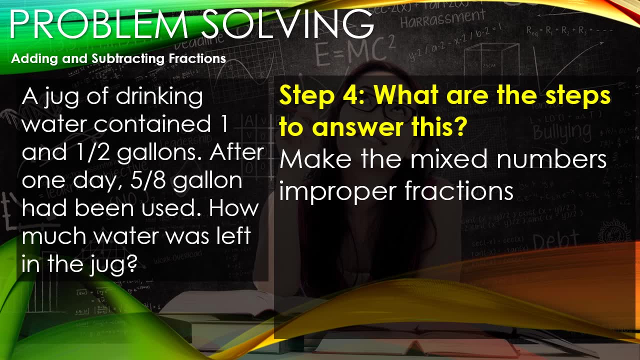 going to set it up one and one half minus five-eighths, so right now you made it to step three, which means that you are over halfway there in solving this problem, so let's go ahead and keep working at it. so what are the steps to answer this problem? so the first step: 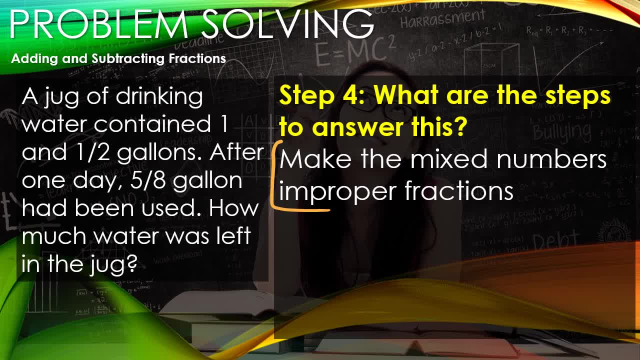 for this one. let's make it easy. let's make all the mixed numbers into improper fractions, and if you don't know how to do that, it's okay, because in the next step we'll show you how to do that. then you can make common denominators and 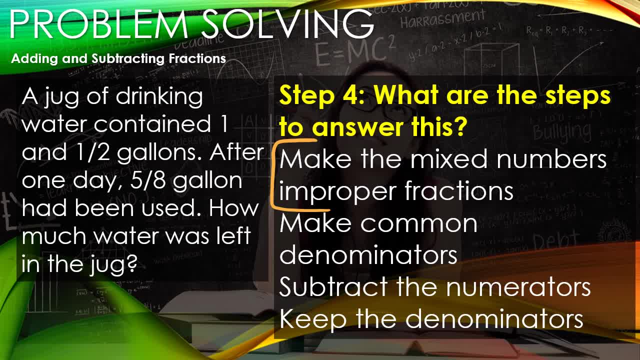 then you can make common denominators, and then you can make common denominators and we're going to subtract the numerators and keep the denominators, and so whatever denominator that we got right here in the step making common denominators, that's the one we're going to use in our final answer. so right now we have it set. 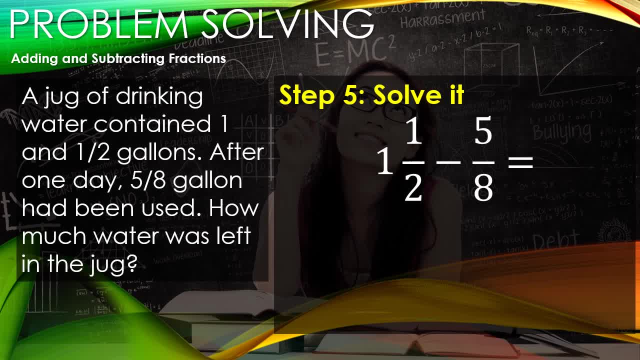 up. let's go ahead and solve it, and so our first step is: let's go to make our mixed numbers improper fractions here. so two times one is two plus one is three. so I have three-halves minus 5, 8. our common denominator is going to be 8, so let's go ahead now. 5, 8. 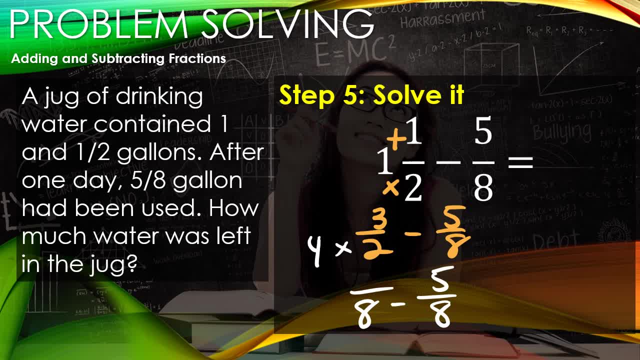 stays the same. so 2 times 4 gives us 8 and 3 times 4 gives us 12. so we're gonna have 12, 8 minus 5, 8. the denominator stays the same. so we ever 8 here and now I'm just doing 12 minus. 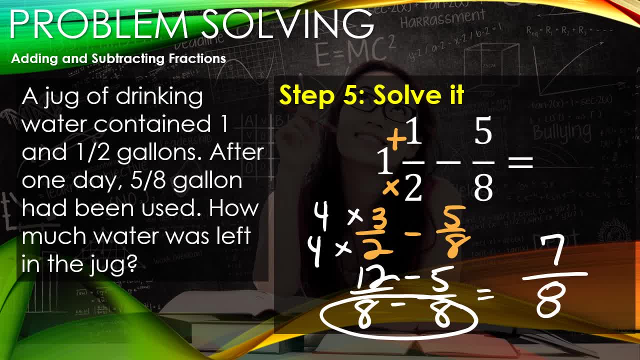 five, that's gonna give us seven. so I can say that how much water was left in the jug? seven, eighths gallons. seven eighths of a gallon was left in this jug. so for your next step, what you're gonna do is you're gonna go into IXL and you have a 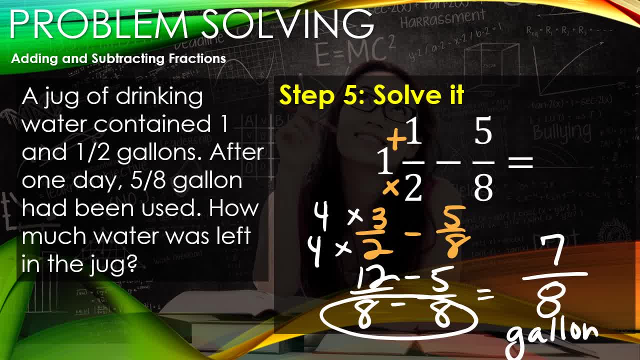 sheet that has ten blank spots in it. so these blank spots. what they're gonna do is that's gonna be where you're gonna show your work for your classwork today. 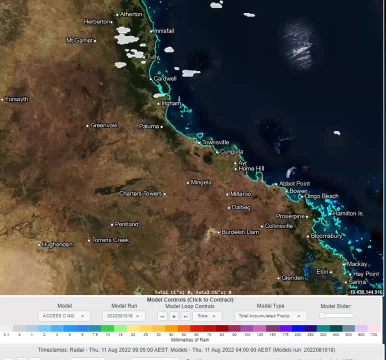 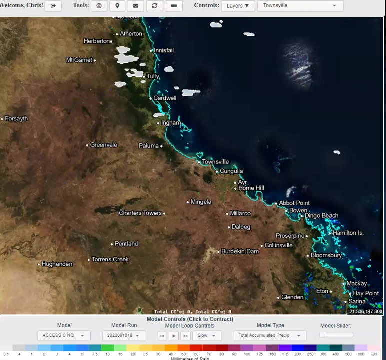 Welcome to tutorial 9 of our tutorial series on how to use the OCC Weather Center. Tutorial 9 probably deals with the most advanced and most powerful tool that we have on the OCC Weather Center. I do warn you, this is not a novice or a beginner tool. This is a sounding tool. So if we 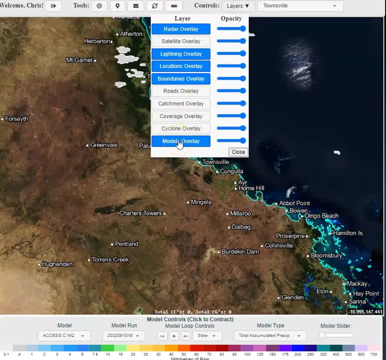 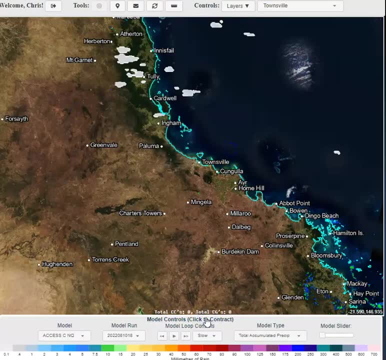 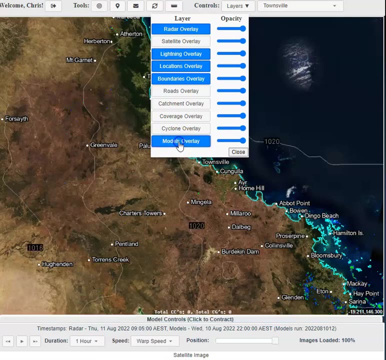 click on layers, we make sure that our models overlay is highlighted or clicked or active. We have our model controls down here, but we're not going to use those for now. What we want to do is, once we activate our models, we want to, once activated, go over here to our soundings. 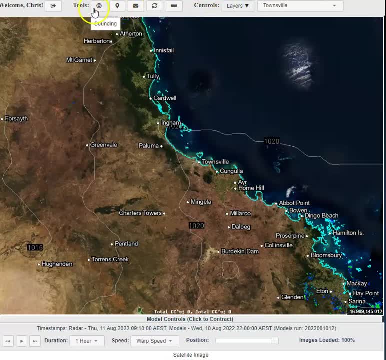 So this is our little target icon, so we can get rid of that layers column, and what we want to do is highlight the soundings. Now, anywhere that we click on the map, what will happen is a sounding will pop up for that particular model runtime. So right now it'll pop up for Wednesday night. 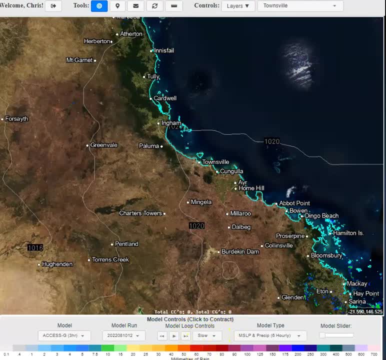 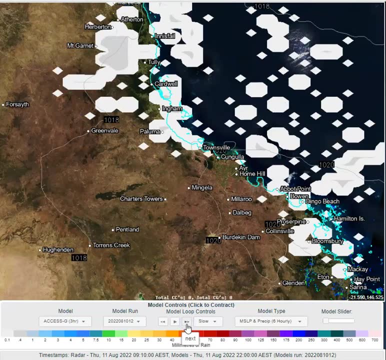 If we take a look here, we can move that model. so we can move that to whatever time frame we want. that encompasses where the model gets to. So, for example, I don't want to look at Wednesday night, I want to look at Thursday afternoon and find out if I'm a chance at a thunderstorm And to do that. 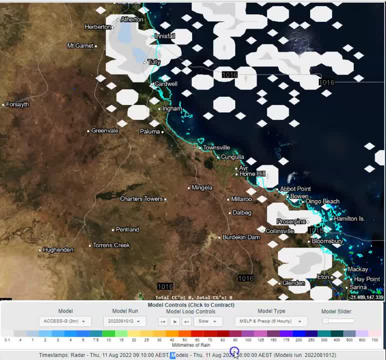 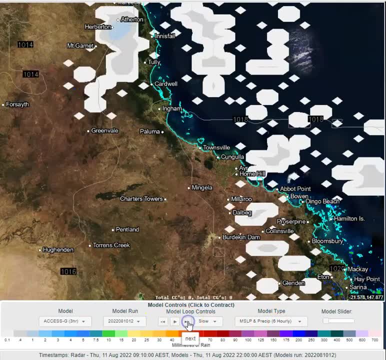 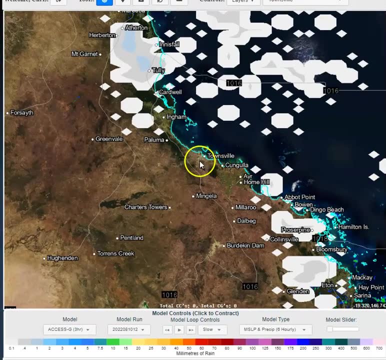 I've clicked on Thursday afternoon on the model run. so models Thursday 4 pm. And then what I've done- and I do that, by the way, just if you take another look. I do that just by moving this along Thursday afternoon. I then want to click on any part, and my little part right here is where I live.